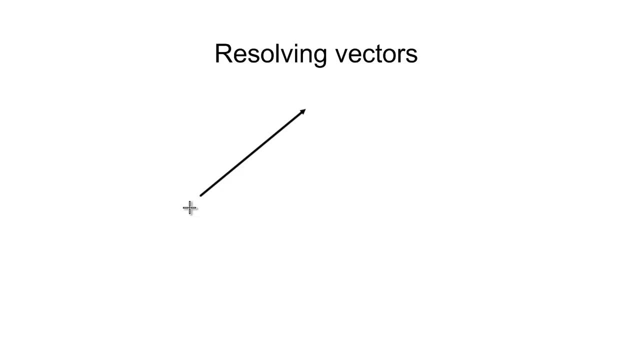 In this video, I'll be explaining how we can resolve any vector into two perpendicular components. Usually, these are horizontal and vertical components. However, it is often asked of us in exams to calculate the parallel and perpendicular components. The methods are identical. we just need to follow the same steps each time. 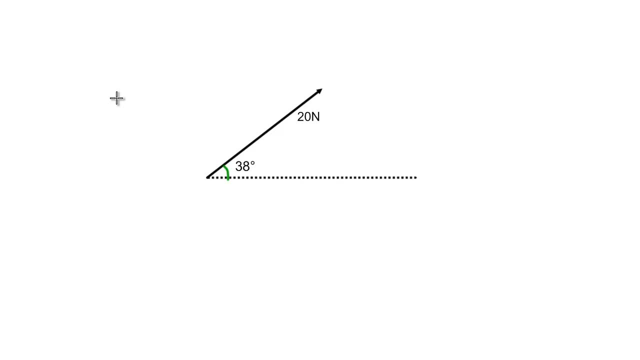 Here is a vector with a magnitude of 20 newtons at an angle of 38 degrees from the horizontal. Let's resolve it into its two components. We can draw our components on. Here is the horizontal component and here is the vertical component. 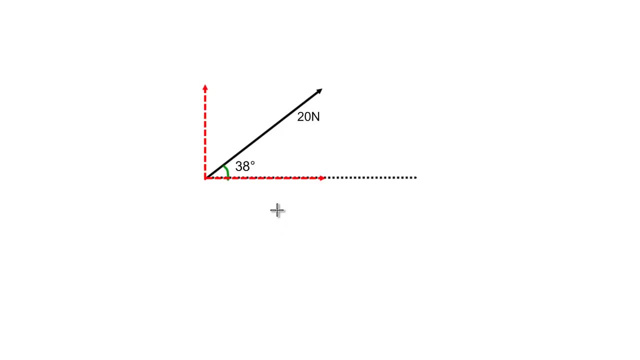 The horizontal component is referred to in your formula sheet as Fx and the vertical component is referred to in your formula sheet as Fy, The component that is touching our angle. this horizontal vector, in this case, is always calculated by multiplying the size of the vector. 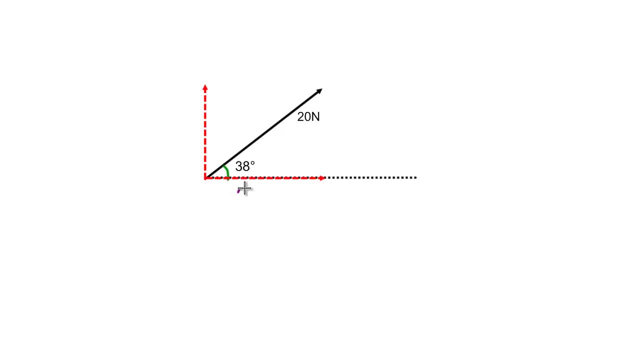 by the cosine of the angle. So in this case the horizontal component will be 20 cos 38, which equals 15.8 newtons. The component of the vector not touching the angle, in this case the vertical component, is always calculated by multiplying. 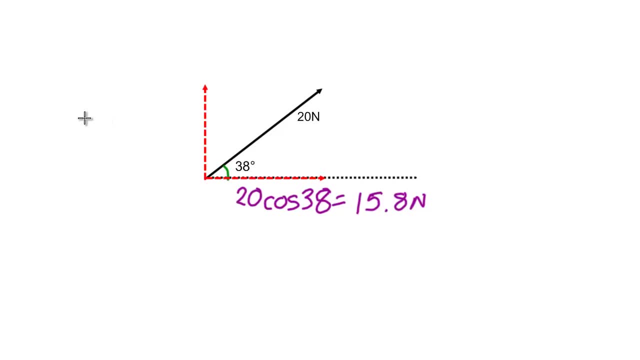 the magnitude of the vector by the sine of the angle, So in this case it will be 20 multiplied by the sine of 38 degrees, which is equal to 12.3 newtons. So there we have one vector divided into its horizontal and vertical components. 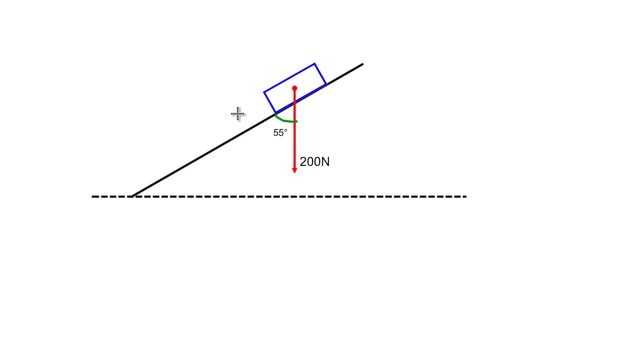 As mentioned at the beginning of this video, the two components that we resolve a vector into do not have to be horizontal and vertical, as long as they are perpendicular to each other. In this example here we have a vector acting vertically downwards. 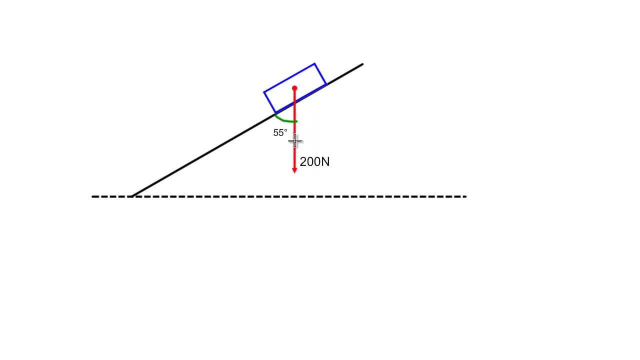 This is the weight of a box resting on a slope, but because it is a weight, it must be acting vertically. The angle between the slope and the direction of this vector is 55 degrees. We can resolve this vector into two components: One component that is acting vertically.